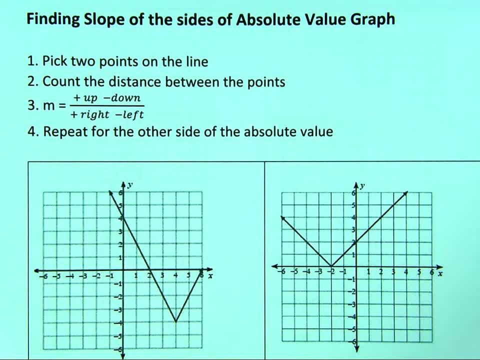 Slope is rise over run. So we're going to pick a point on our graph, We're going to pick two points. We're going to go up and over until we get to that point. The next, another point on the line. 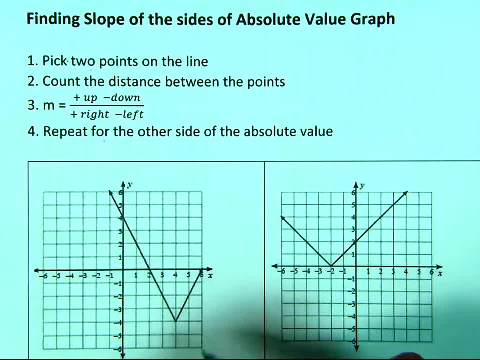 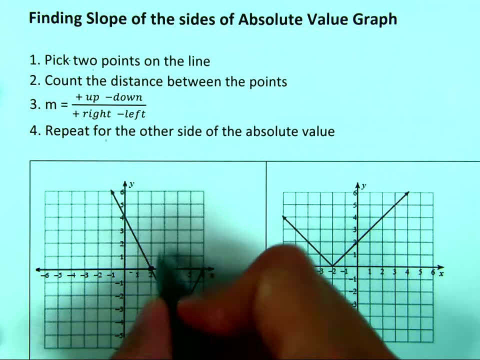 And then that will help us know what our slope is. So here we go. So we're just going to pick any old point here. I try to pick it where it crosses the grid so that we can count easier. If you pick it in here it's hard to tell. 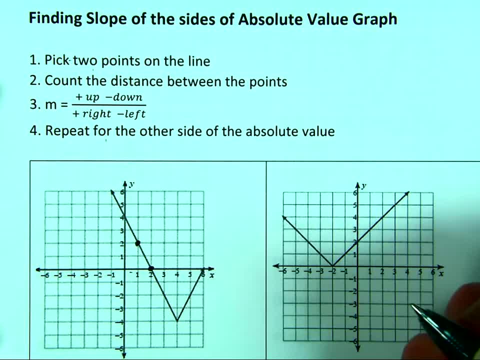 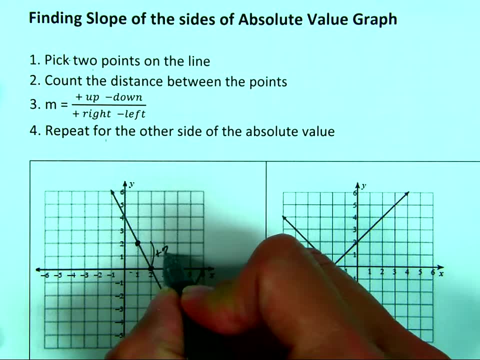 So we're going to pick that point. and then I see, right here it crosses the grid too. So on the left branch of the absolute value I would be going up two and left one. You've got to remember that up and right are always positive, down and left are always negative. 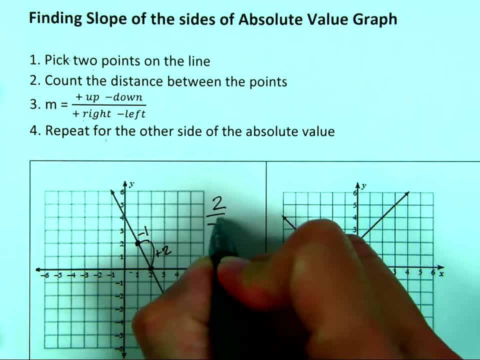 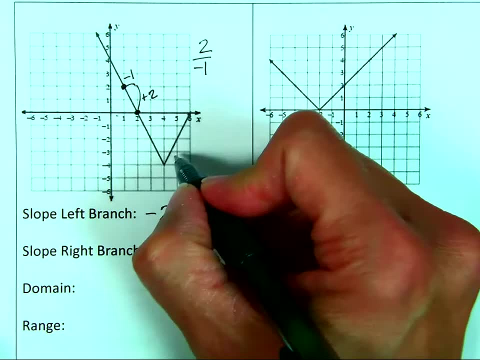 So up two, down negative. So if I pick negative one, the slope of the left branch then is negative two. Now I'm going to find the slope of the right branch, so I'll just pick these two points. 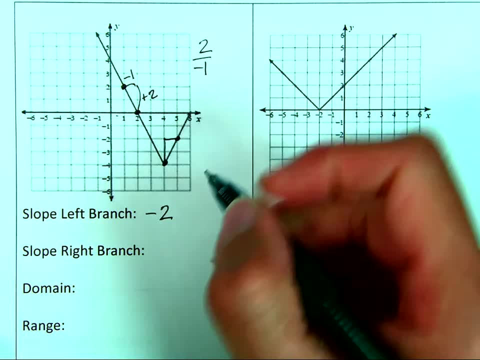 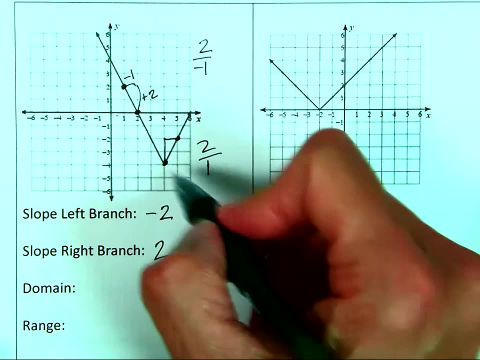 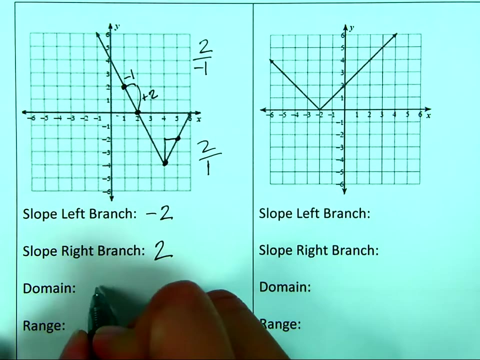 Look, it goes up two over one. so the slope is two over one, which means the slope is positive two. Now you see these little arrows on the absolute value sign. they go forever left and forever right. So that means that my domain is all real numbers. 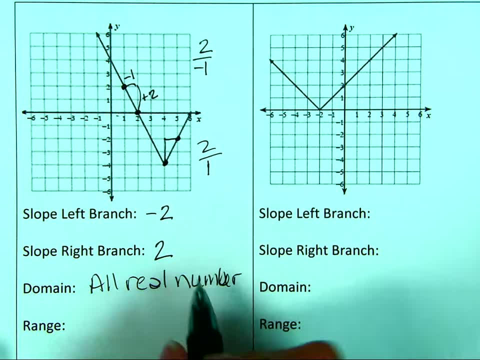 Because it's always real, It's always going to be going left and it's always going to be going right, And so domain is values of x, the x-axis goes up to right, So it's all real numbers. Now the range you'll see from this point: it goes up forever, but it doesn't come down forever. 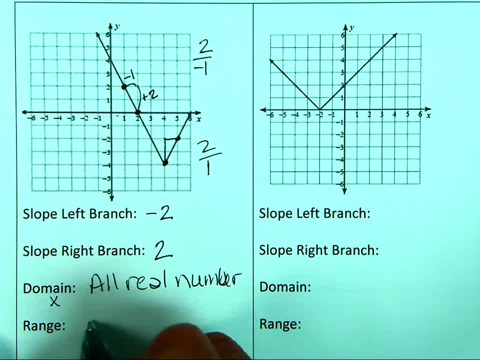 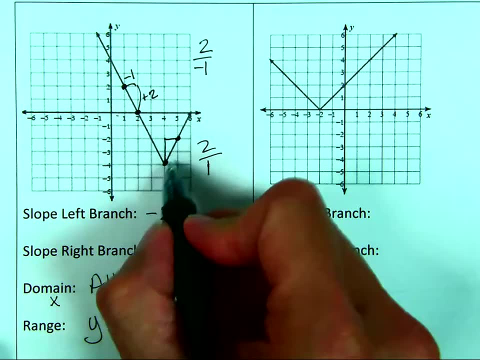 So our range actually has a starting point. looks like it's negative four and range is y, And so y is going to be anything that's greater than or equal to whatever that vertex is. That's that low point right there, that starting point. 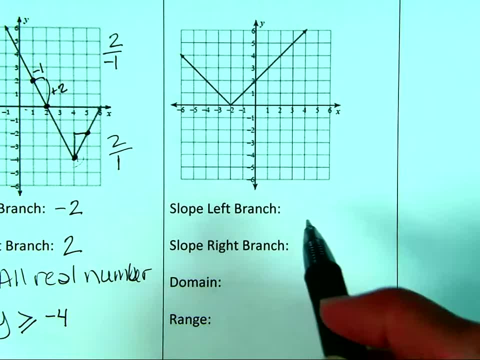 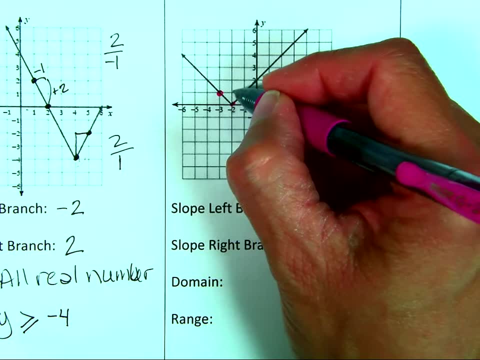 So that is that one. Let's try another one. Left branch, So left branch. we're going to pick two points. We'll start at the vertex. Looks like right. there's another point, That's up. one left one. 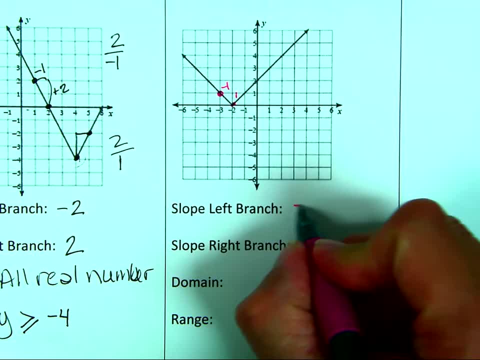 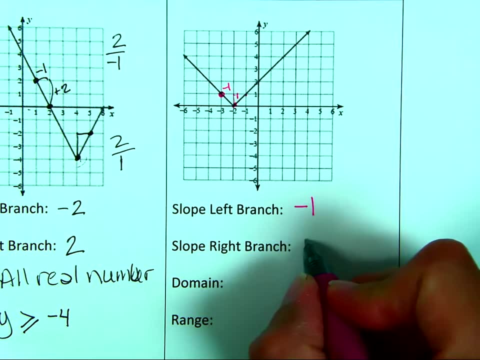 Up and left means one over negative one, which means my slope is negative one. If I pick it on the right branch, I'm going up one right one. So that's a one over one. So my slope is one. 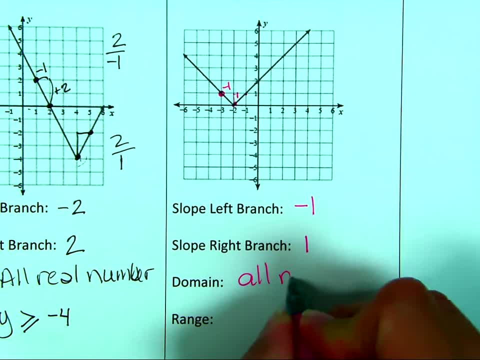 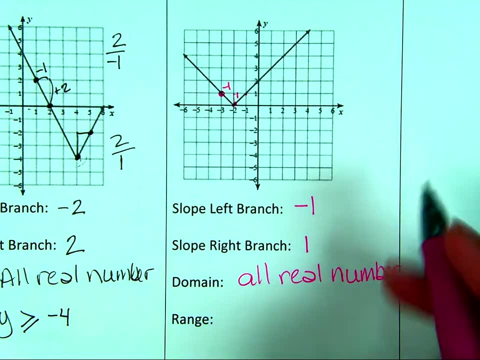 Again, my domain for absolute value is going to be all real numbers, Because it goes left forever and right forever. My range, however, is going to have a starting point, Because it starts right there and then it goes up forever. 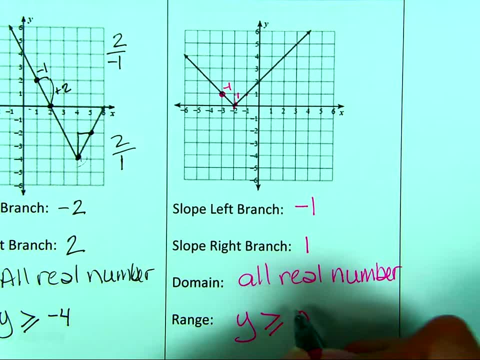 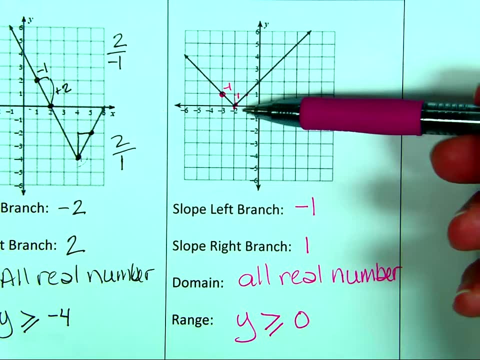 So it's going to be greater than or equal to zero. Keep in mind that we want the y value, So this is the y value. It's not the x value, which is negative. two, It's the y value because you're going up and down. 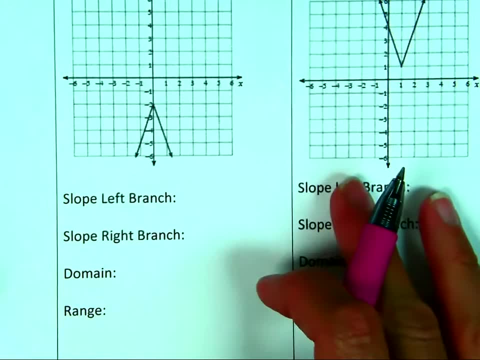 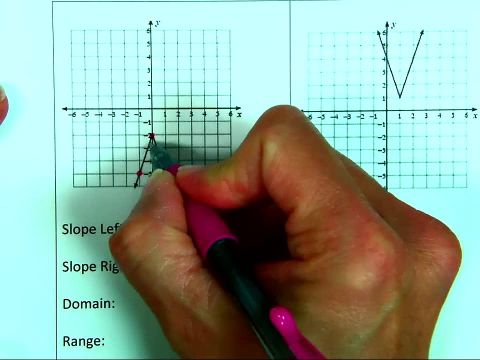 Okay, let's try a few more. Two more, Okay. so let's find the slope. So here I'm going to start and it looks like it ends right there. So that's one, two, three. It's down three and a left one. 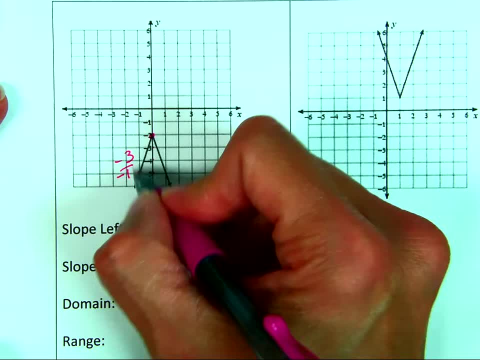 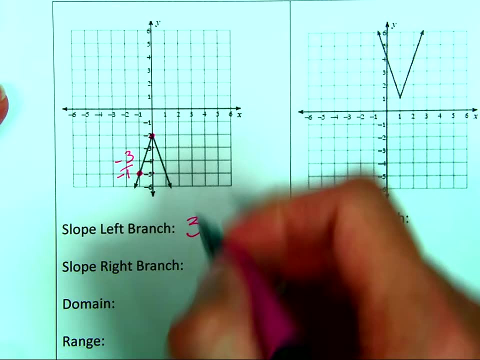 Down three and left one. for my left branch, Down three and left one would just be a positive three. And now for my right branch, it looks like it's down three and right one. Down three and right one would be a negative three. 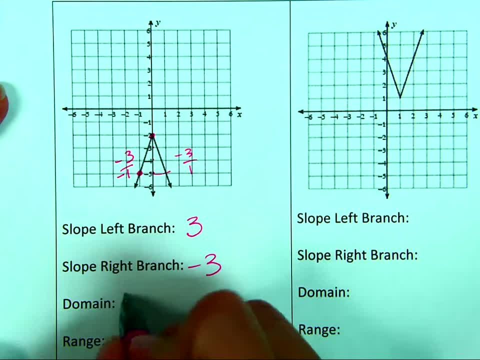 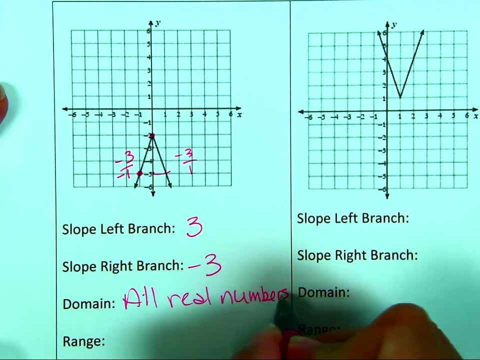 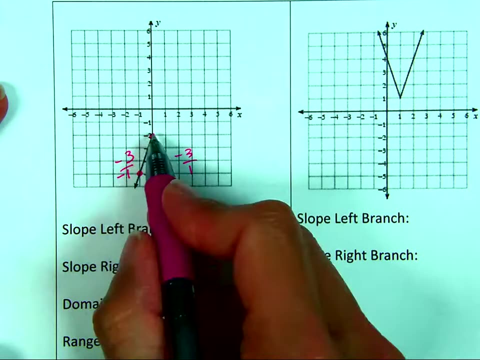 Again, the arrows are going left and right forever, So you should know what that means by now. All real numbers for my domain And then for my range. it looks like it starts here and goes down forever. So now my y is going to be less than or equal to that number, negative two. 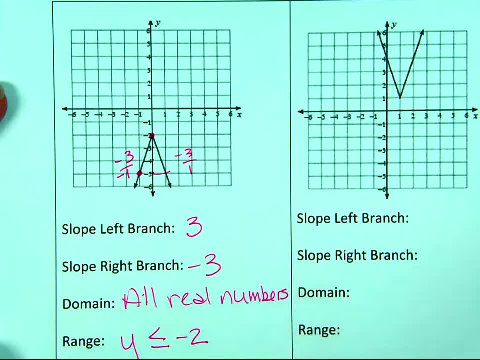 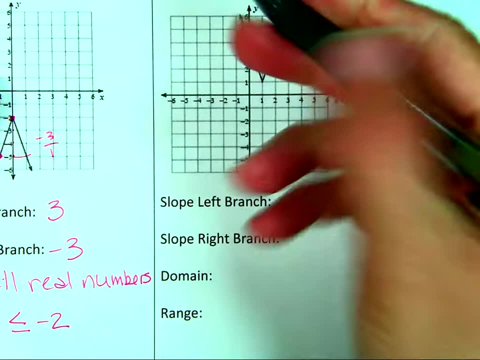 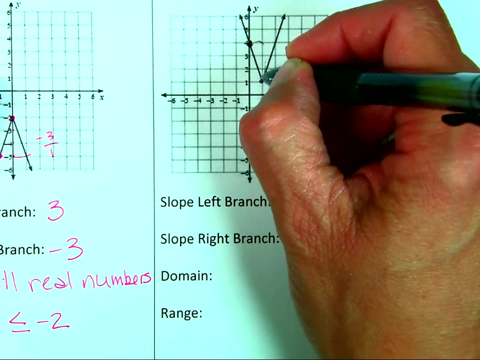 Not greater than because it doesn't go up, It goes down. All right, last one. So you can see here that my left branch. if I go right here it looks like it's up three: right one, I mean left one. 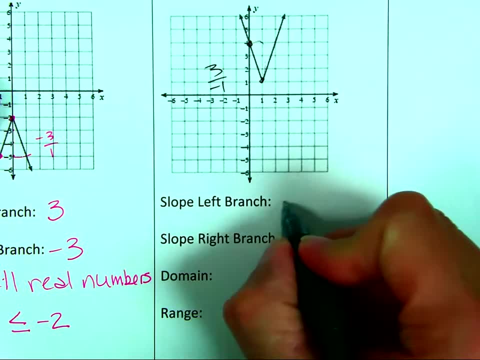 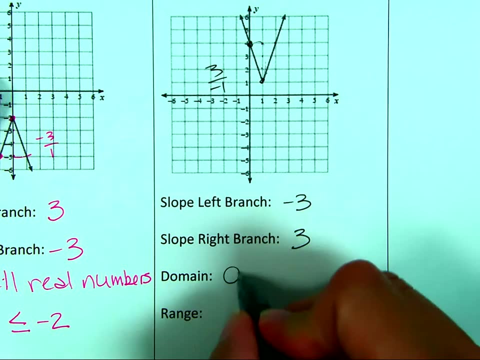 Up three left one, So that's a three over negative one. That's a negative three, And then one, two, three, one Looks like it's a positive three on that side, My domain again would be all real numbers. 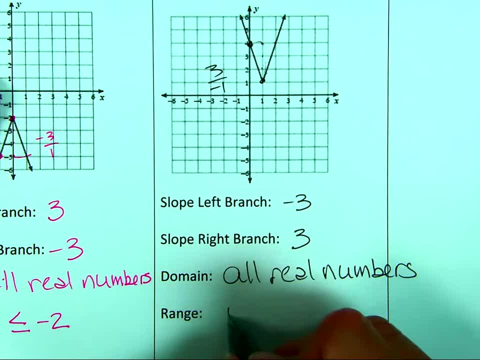 And my range starts right there and it's going up, So it's going to be greater than or equal to one. So I wondered if you noticed that the slope of the sides of the absolute value of the absolute value, of the absolute value.